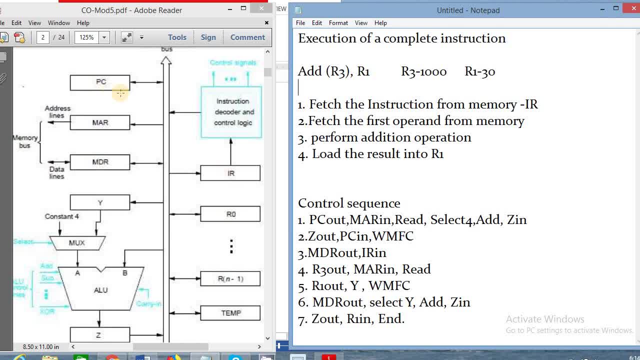 what instruction we want to execute. the address will always contain in program counter And MAR contains the address register, MDR. all the data we are storing in MDR register, Instruction register. all our instruction is storing in instruction register And this is our general purpose register: R0, R1,, R2, R3, then up to R and minus 1.. One temporary register is there. Y register is there. Multiplexer: two input multiplexer: One input is 4,, constant 4, and 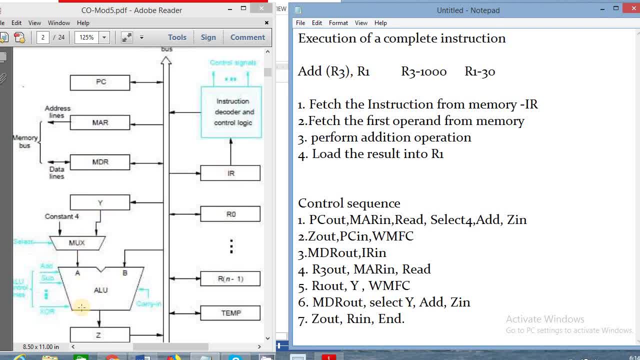 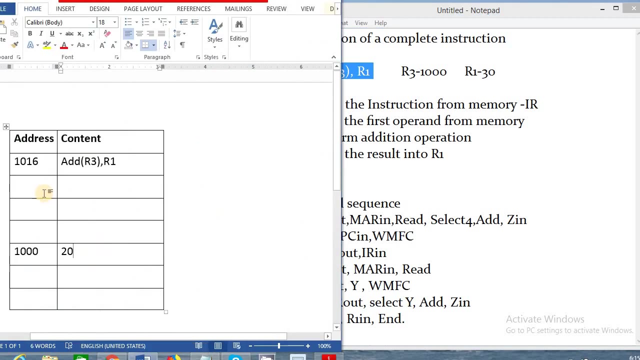 another input is output of Y register and ALU. Output of ALU is always storing in Z register. So this is our architecture. based on this, Let's see how to work on this instruction, So how to execute this instruction. The first step is pass the instruction from the memory, So this instruction is stored in memory. I will show you one diagram of memory, just see here. So this is my instruction. It is stored in my 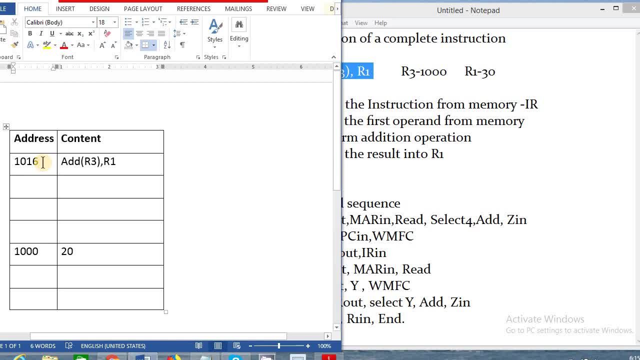 so this is the address location. assume this is address location. it is short and another location here: thousand. it contains some value 20, so let's see what happened here. so where this address I can get. I can get this address from my PC. that is our program counter contain the address. so I am taking the program. 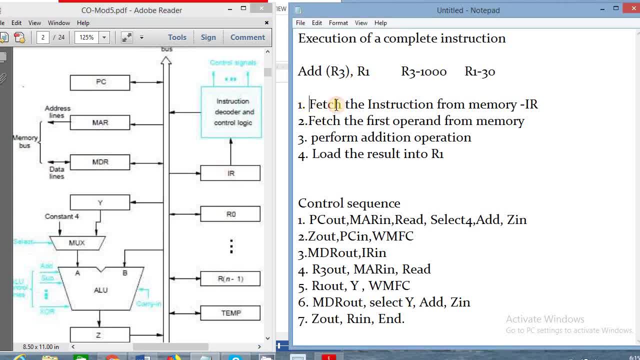 counter address. then I am taking the data from the memory. that is what called fetch the instruction from the memory. so after taking this instruction from the memory, I will store this instruction in IR register, because currently executing instruction, storing in IR register, next fetch the first operand from the memory. so 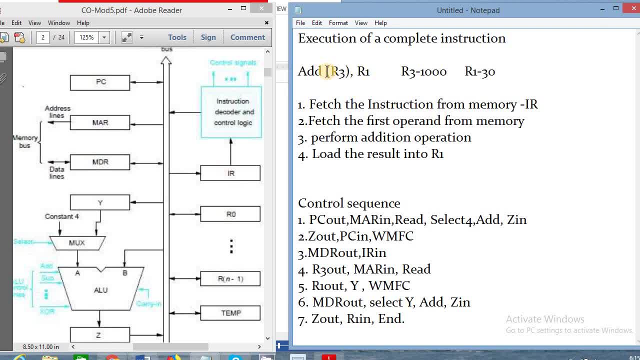 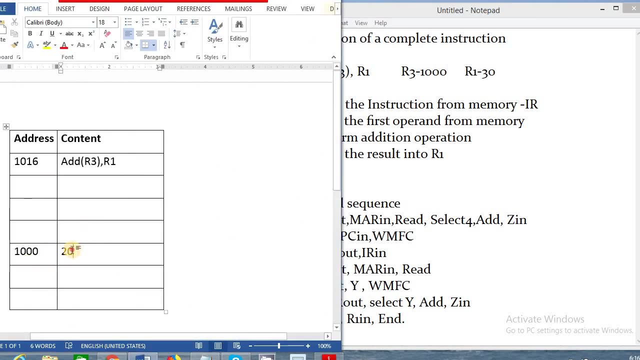 this is my first operand so this parenthesis indicates it is a pointer. so pointer means what assume? R3 contain an address thousand, so R3 not contain some data. R3 contains some address location so when we are seeing that address location, the main memory we can see some data is there. that is 20 in our example, so that 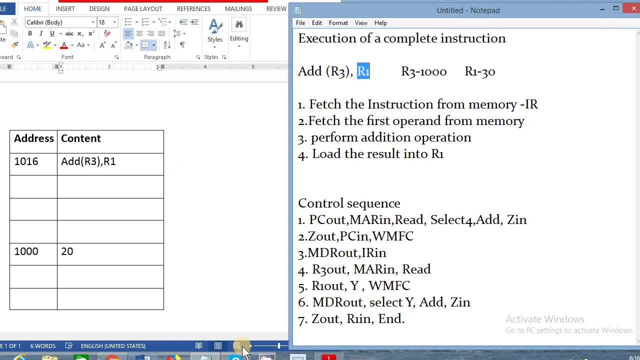 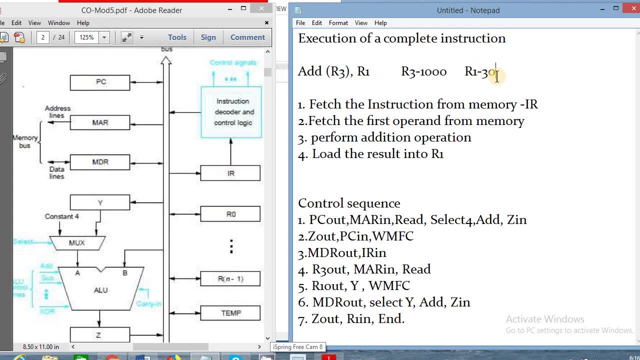 20. we are adding with R1 register. so R1 register in our figure it is: comes here R1, R3 comes here. R1 contains some data. for example, R1 contains 30, so this 20 should add with 30 and the result will store in R1 now. so we 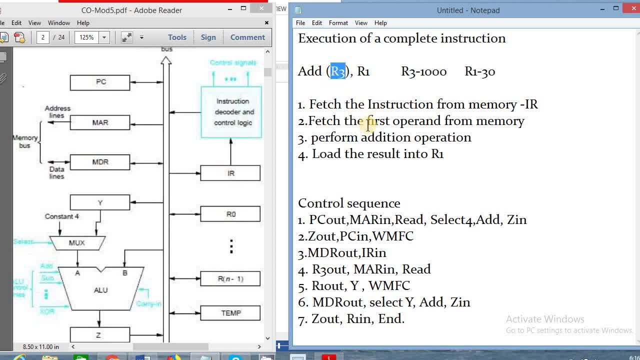 should fetch the first operand, R3. that is in the main memory. we should take that data and then perform the addition. then the result should store in R1. so how to write the control sequence for that? so I am writing like this: where address of this instruction is stored, it is in PC. so program counter out: I am. 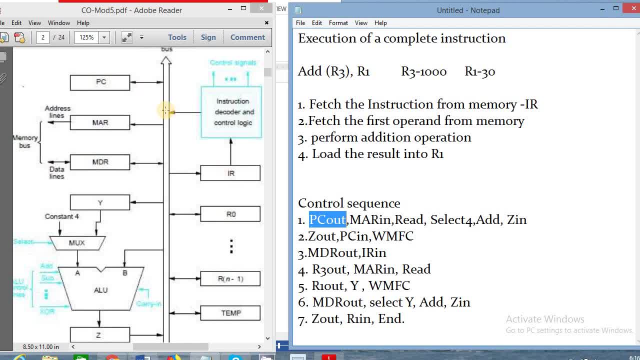 taking the address from program counter from here. that address I am storing in MIR, that is MIR in. I have written MIR in, so address is containing MIR register. then here through the memory bus the address is sending through memory, so memory is reading that data. so read control signal issue: reading the data. 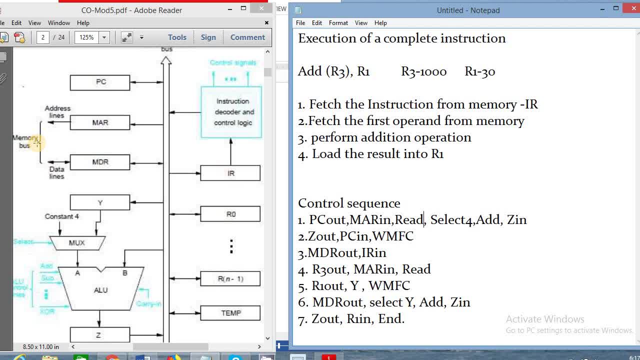 So reading will take some time, Assume that it will take some time. So in between, another operation I am doing- I am going to increment this program counter. So why should I increment the program counter? So next instruction is stored in address of the next instruction is stored in program counter. So I should increment the program counter. 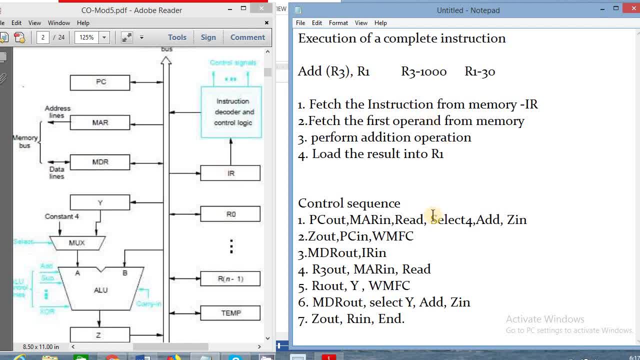 So to increment the program counter in 32 bit address system we are incrementing by 4.. So select 4.. So where I am selecting 4 in the multiplexer 2 input is there 4 and Y. So I am selecting 4 here. That 4 will come here in A And PC content will come to B. So add PC content with 4.. So result is stored in Z. Then that result will store in PC, So like that I can increment the PC. 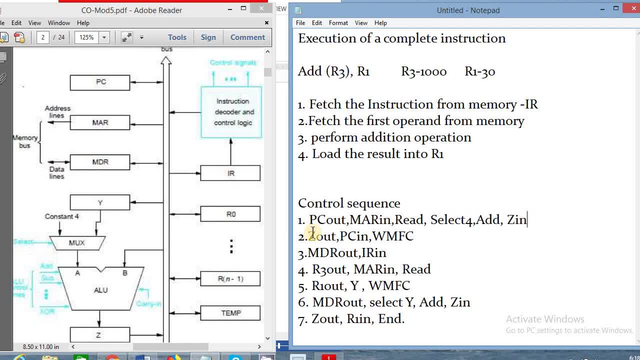 So select 4, add: storing in is a register and is a doubt will store again in pc in now pc incremented. now what is w m of c that is called waiting for memory function complete. so memory function complete is a signal from the memory. then what more operation we are doing here? read operation we are reading, so what? 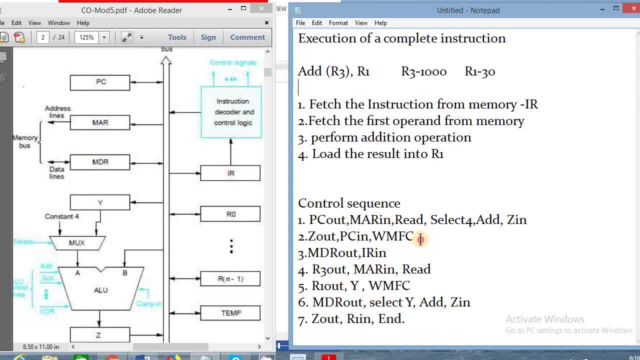 we are reading our instruction, we are reading from the memory. so when this reading operation is completed, memory will set this memory function complete signal. so we are waiting for that signal, that is w, m of c. so when this reading operation completed, this instruction, our instruction from the memory will store in data register. so here, through the memory bus, our instruction will come. 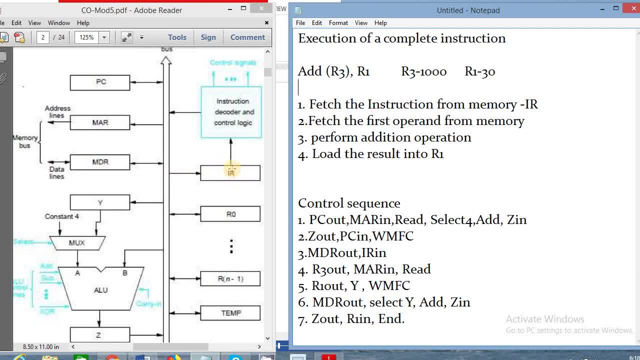 to data register. from the data register it will store in instruction register. so currently executing instruction, store in instruction register. that is mdr out, ir in. now what happens when we are executing this insertion? what we should do next: fetch the first operand from the memory. so what is first operand are three is a pointer it contained tangled, then that thousand. 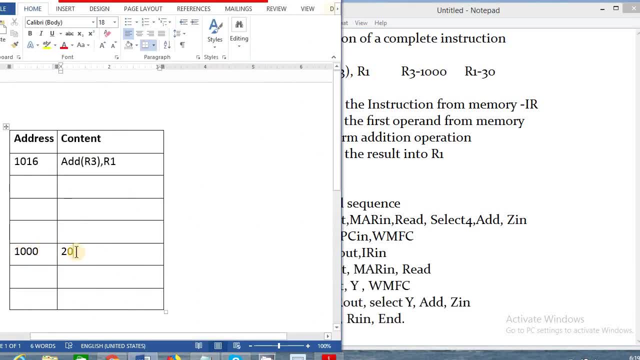 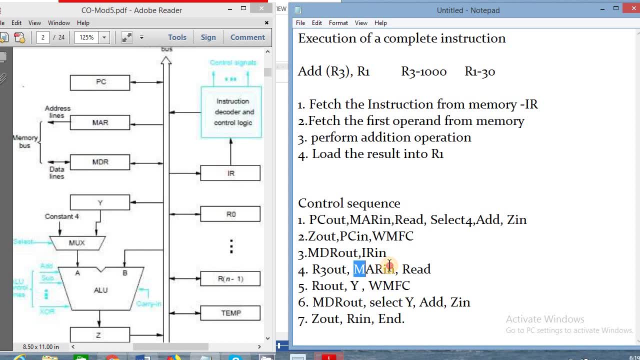 address location contain some data. we already seen that thousand others location contains some data. so that data we have to face. so what we should do? our three out: that is thousand. that address we are storing in America's. so here our r3 comes from this R 3 that address is storing in a male. 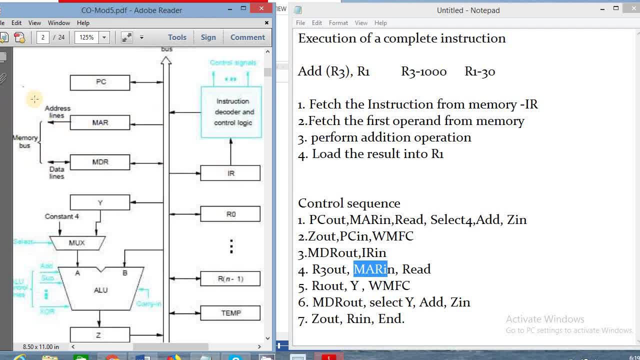 register from the mirror address is sending to memory through the memory bus and data is reading- and that's what i should read control signal here and we are waiting to read operation to complete. when the read operation is completing the data will come in. come in mdr register. that mdr data we are taking out. 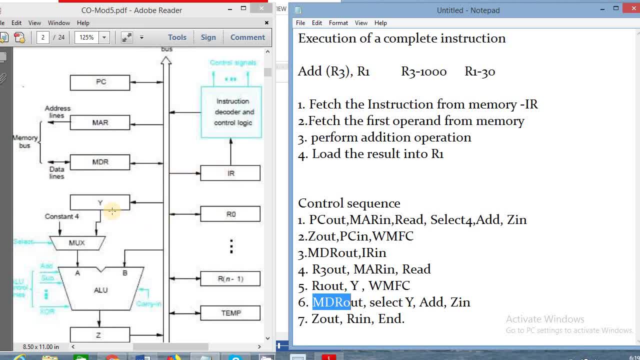 and that will store in y register temporarily. in between, one operation is happening. we need the second operand, r1. so r1 out, that is a processor register. it is here r1 register and uh, this r1 data we are storing in y register temporarily. y in, that's what i've written here. y. 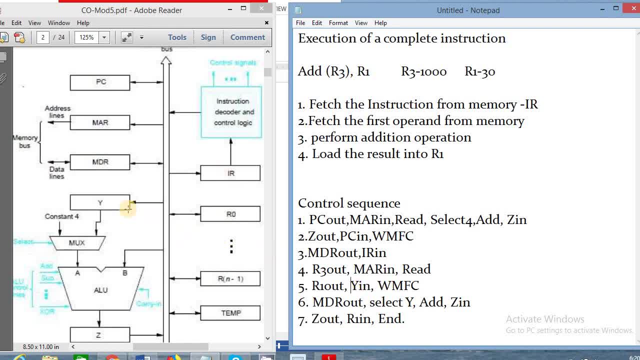 in. so r1 data from here is stored in y register. so r3 data out mar in reading operation waiting for memory function to complete. when the memory function complete, mdr out data will come to md r register. so first operand is available in mdr. second operand is available in y register. so we 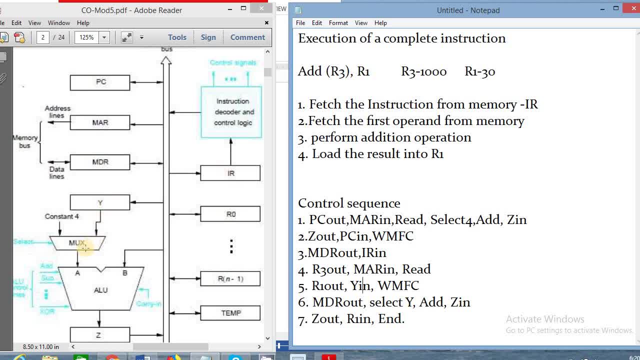 should add here. so from my register to the multiplexer. the second operand comes here. first operand from mdr. it comes in point b. so we are adding these two, that is add and z in. result is storing. in is a register. from this register it will store in r1.